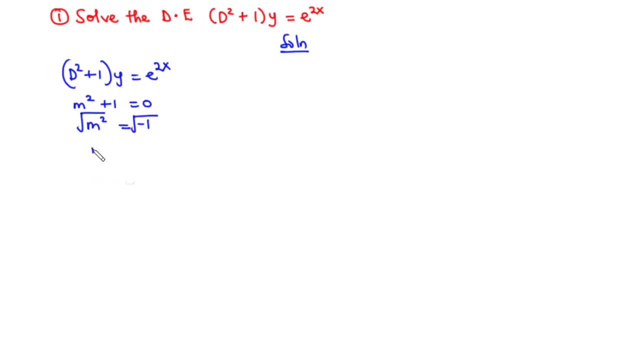 And then we transpose 1 to the left-hand side, And then we transpose 1 to the right-hand side, And then we transpose 1 to the right-hand side, And then we transpose 1 to the right-hand side, And then we take the square root of both sides so that we have m equals plus or minus i. 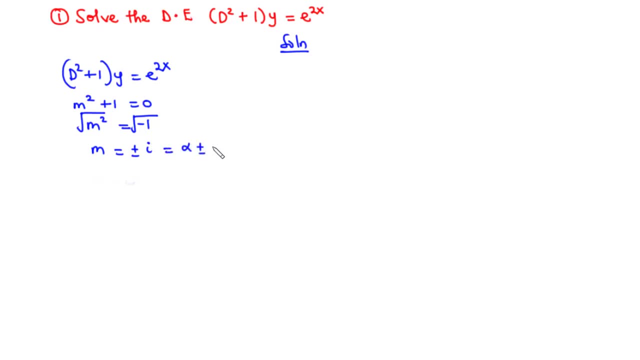 Now, comparing that to alpha plus or minus i beta, you realize that we have alpha equals 0.. And then we have beta equals the coefficient of i, which is 1.. Therefore we have the complementary function yc equals e to the power alpha times x into bracket c1.. 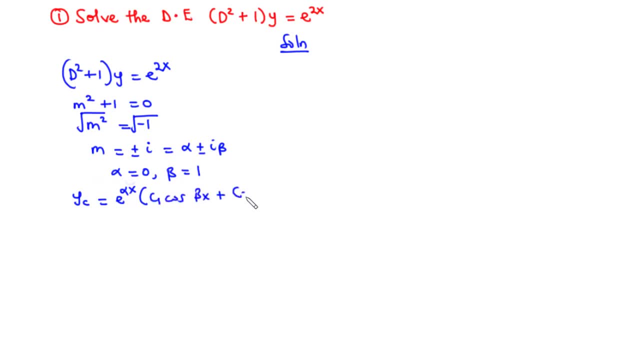 So we plug in the values of alpha and then beta Alpha is 0.. 0 times x is 0.. e to the power 0 is 1.. So we have 1 times c1 cos, 1 times x is x. So c1 cos x plus c2 sin x. 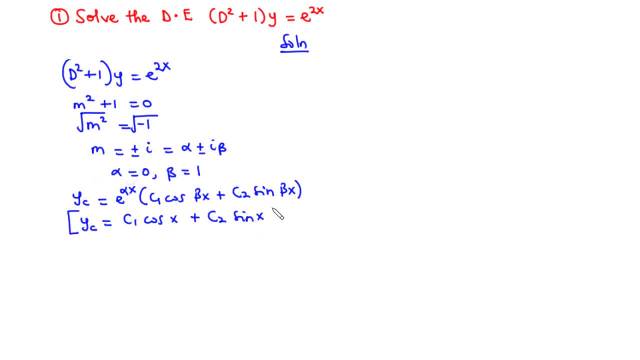 So this is the complementary function. Now let's try to find the complementary function. Now let's try to find the particular integral. So for the particular integral, we have j of x, the function on the right-hand side, to be equal to e, to the power 2x. Now this: 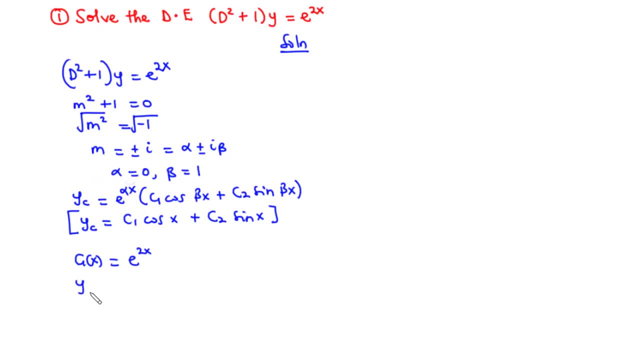 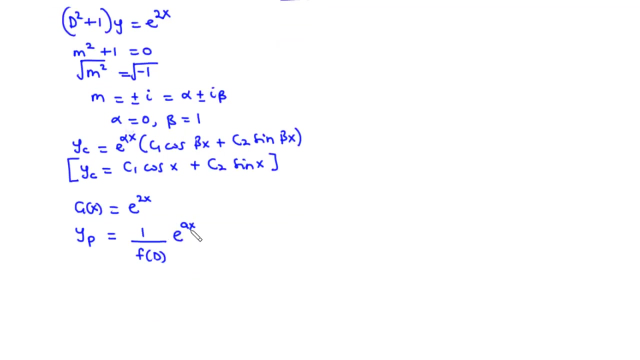 is an exponential function. So we have the particular solution or the particular integral. yp equals 1 over f of d times e to the power ax. Now if we find the particular integral j of x is an exponential function, Then basically you are going to substitute or: 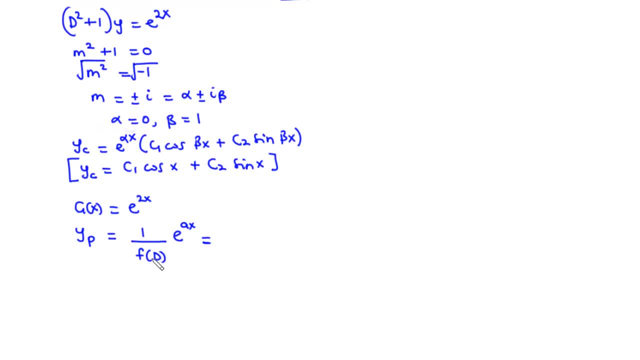 you are going to plug in the value of a in here into the polynomial function of the d operator, So you have 1 over f of a times e to the power ax. Notice that this is valid so long as f of a is not equal to 0. So comparing this to that, you realize that 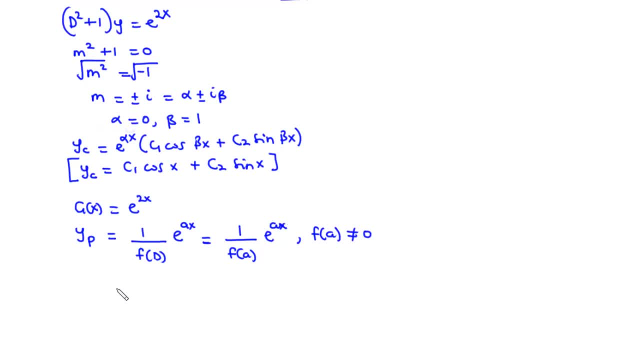 we have the value of a to be 2.. Therefore we have yp equals 1 over Now f of d is what we have as d square plus 1.. So we plug in a equals 2 so that we have 2 square plus. 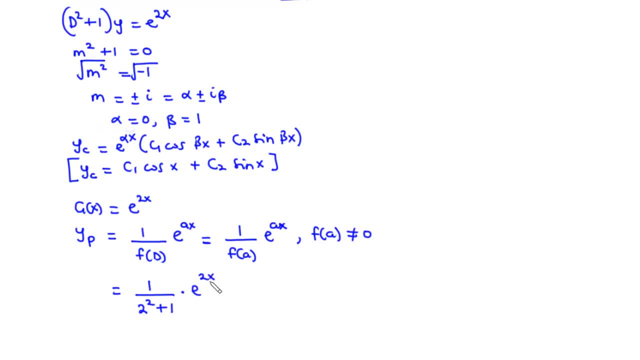 1 times e to the power 2x, So this becomes 1 over 5 times e to the power 2x. This is called The particular integral. Therefore we have the general solution, giving us yc plus yp and that is equal to. We have c1, cos x plus c2, sin x plus 1 over 5 e to the power. 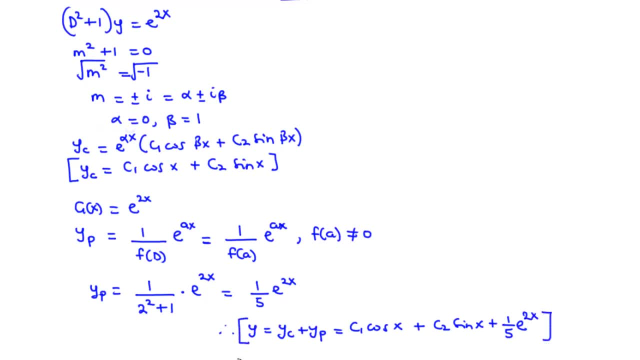 2x. Now let's try example 2.. So we have d into bracket d minus 1 times y equals 5.. So let's try to solve this. So we have d into bracket d minus 1, all times y equals 5.. So for this we have to generate the auxiliary equation. 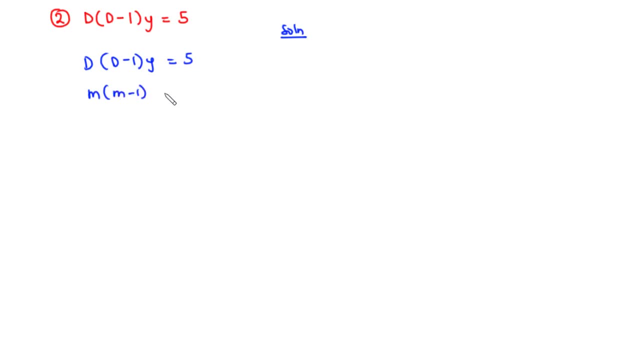 So we have m into bracket. m minus 1 equals 0, and this is m1 equals 0. And then we have m2 equals We transpose negative 1 to the right-hand side So that we have 1. Therefore we have the complementary function. 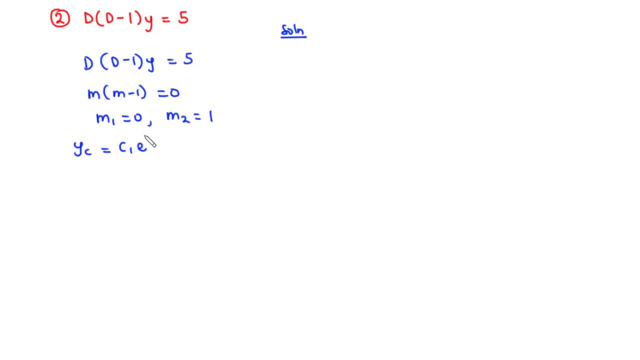 Equals c1 e to the power 0 times x, Plus c2 e to the power x. So 1 times x is x. Therefore we have yc, yc to be equal to e to the power 0 is 1. So 1 times c1 is c1. 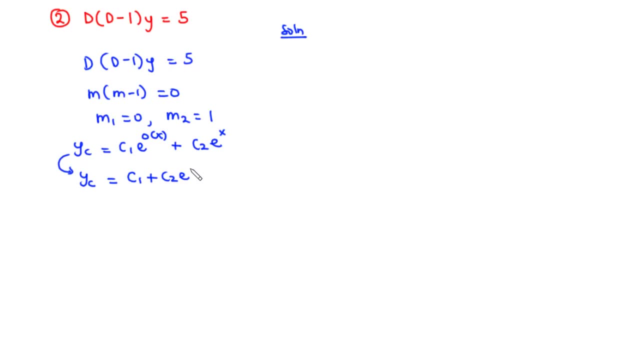 So we have c1 plus c2, e to the power x. This is the complementary function. Now for the particular integral. We have g of x to be equal to 5. Now, this is a constant, or, better still, a polynomial, Where the value of x has a degree of 0. 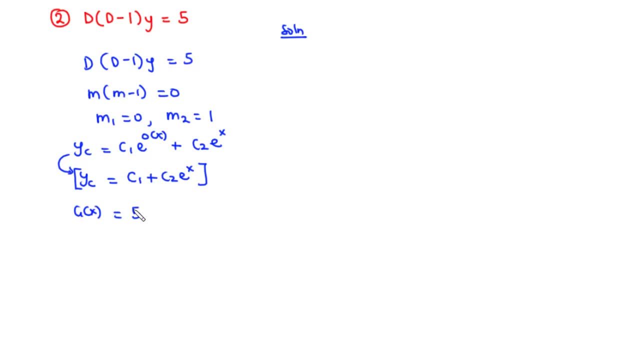 So x to the power, 0 is 1, And then 1 times 5 is 5. Now, so long as we have a polynomial, Then we have: yp equals 1 over f of d And then times the function on the right hand side, And then, because we have a polynomial, 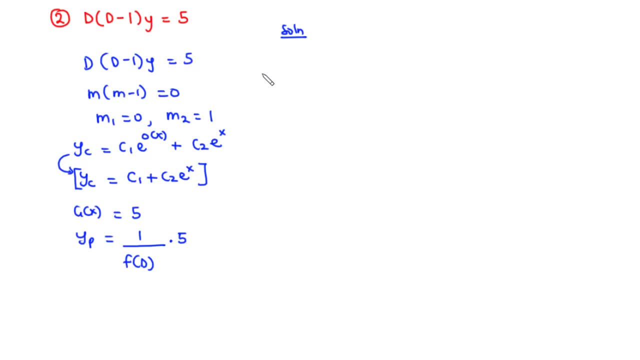 We should be thinking of either of the two expansions, So we can either have 1 over 1 minus d, Which is equal to 1 plus d Plus d squared Plus d cubed, And so on and so forth, Or, better still, 1 over 1 plus d. 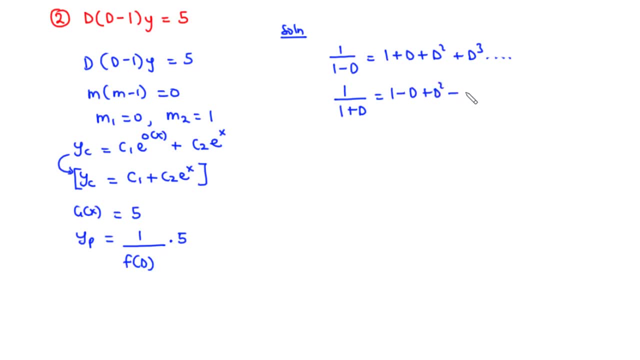 Equals 1 minus d Plus d, squared minus d cube, and so on and so forth. now we can express this as one over. now f of d is giving us d into bracket d minus one. so we have d on the outside, and then d minus one, and then times five. now we want to make sure that one is positive, we want to make sure that one is. 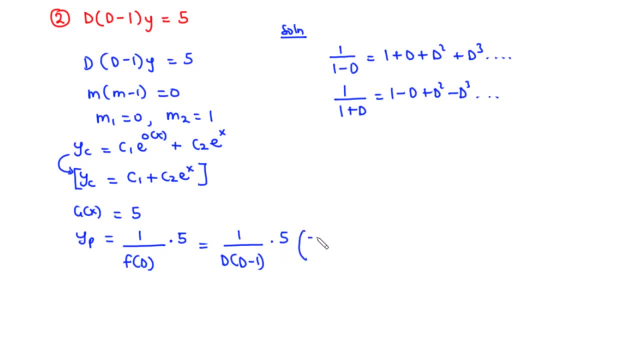 positive. so we are going to multiply top and bottom by negative one. so when we do that, then we have negative five divided by d into brackets. this negative affects the d here, so we have negative d and then it affects this and then we have positive one. now we can interchange. 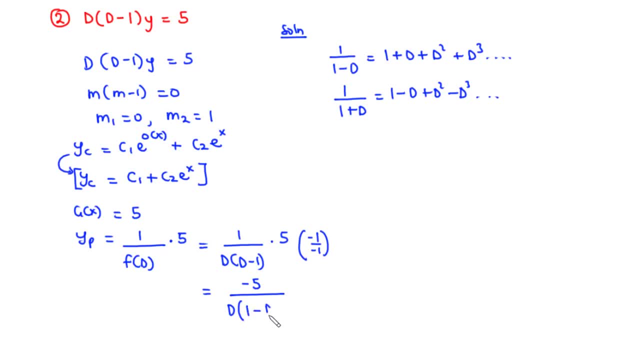 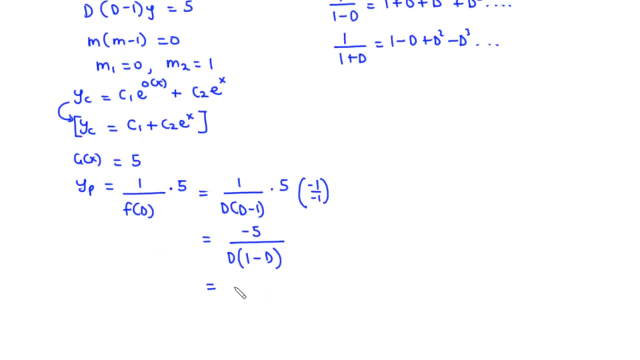 the positions so that we have one minus d. so the next thing we are going to do, the next thing we are going to do is we are going to have negative 1 over d, negative 1 over d, and then we try to input the expansion 1 over d minus 1. 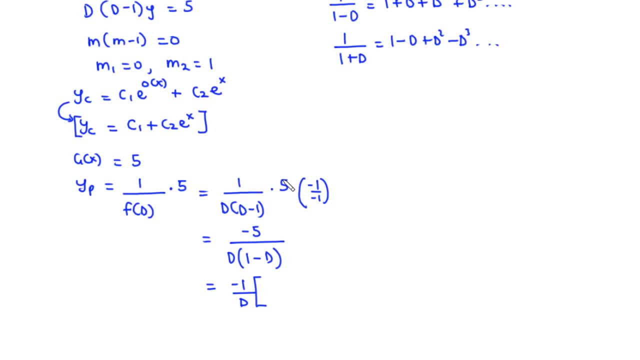 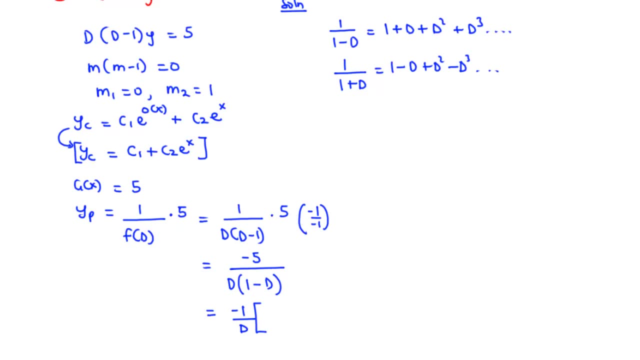 now you realize that here we have a constant. okay, so we are going to focus on only the first value, because here the exponent on x is 0. that is why we have x to the power. 0 equals 1, and then 1 times 5 is 5.. now, if we have 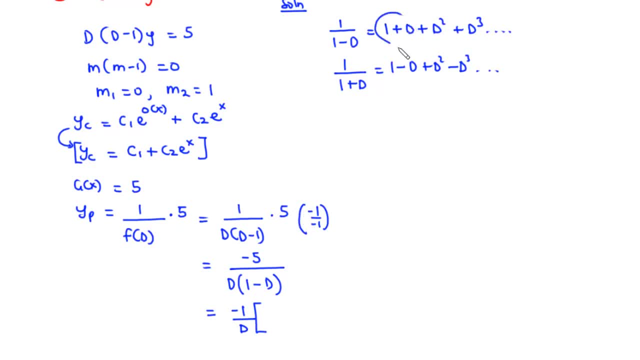 had 5x, then we focus on the two values, because this time we have the exponent on x to be 1- yes, so usually that is how it is done. so we focus on only the constant, which is 1, and then we have the function 5. 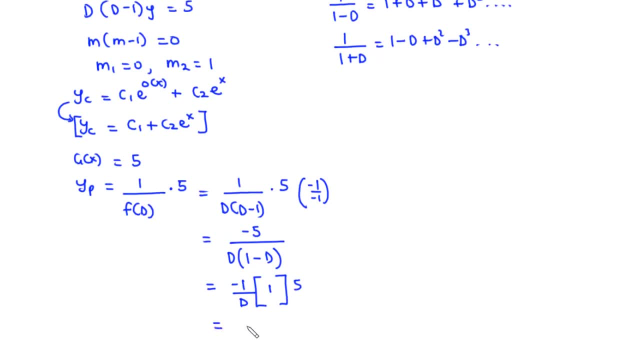 so we are going to have negative or, better still, we have 1 over d, 1 over d times negative 5. now, in the first lesson on the operators, with regards to first order linear differential equations, we said that if you have 1 over d of a function f of x, then basically that is equal. 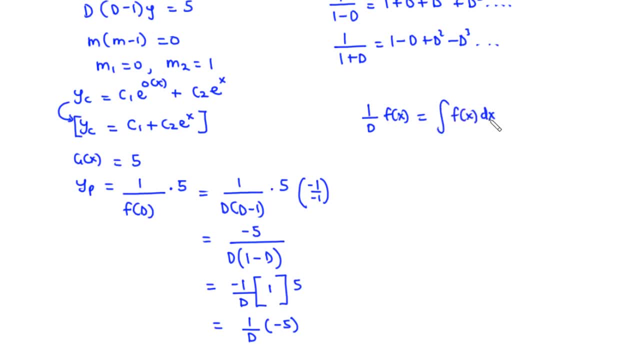 to the integral of the function f of x with respect to x. so in that same case we are going to have this to be the integral of negative 5 dx, and that is simply negative x, 5 x, negative 5 x. so that is yp. notice that we ignore the constant of integration. so we have 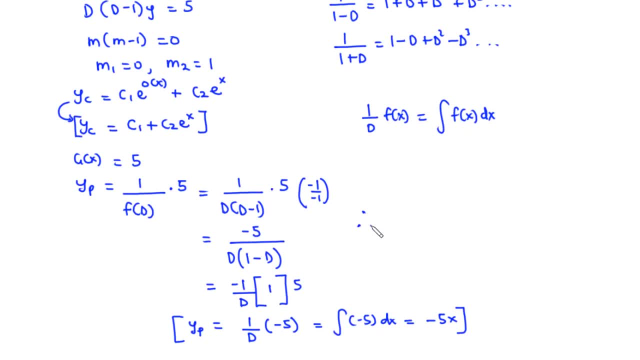 negative 5 x. therefore we have the general solution, which is y equals yc plus yp. you have yc to be c1 plus c2, e to the power, x minus 5 x. now let's move on as we solve the third example. now let's solve example 3. 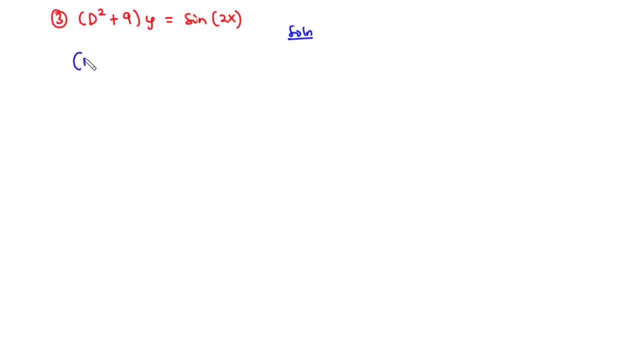 so we have d square plus 9. all times y equals sine 2x. so first we have the auxiliary equation giving us m square plus 9 equals 0. we have m square equals negative 9. we take the square root of both sides and then this can be simplified as the square root of negative 1 times the. 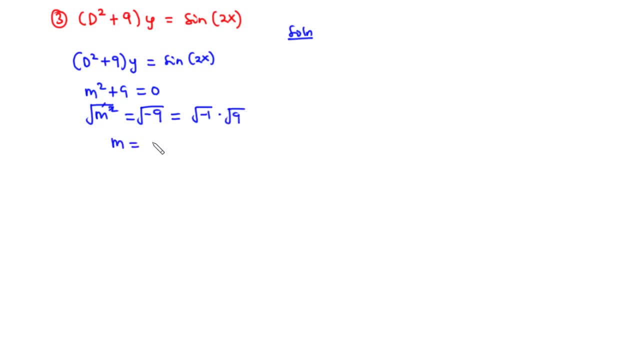 square of 9, so we have: m equals plus or minus. i times 3, so this is a plus or minus 3 i so we have: this is to be equal to alpha plus or minus. i beta and then you realize that we have alpha to be 0.. 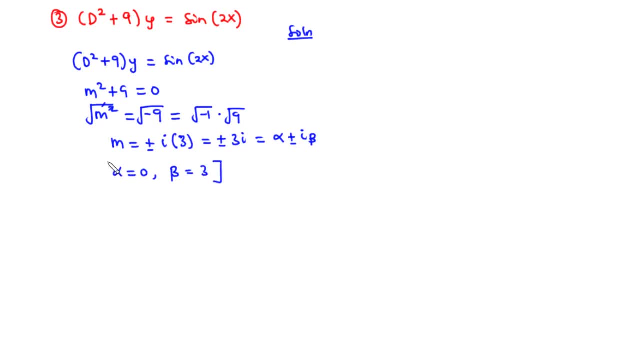 and then we have beta to be 3. therefore we have the complementary function equal to e to the power 0 times x, so that is 0, and then e to the power 0 is 1, so we have 1 times c1, c1, cos 3x plus c2 sin 3x. this is the complementary function. now for the particular integral. 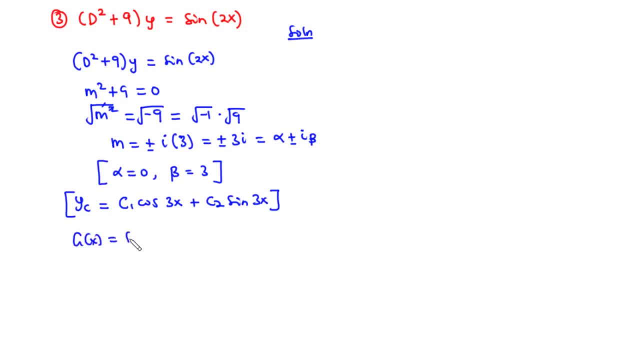 we have g of x giving us sin of 2x. now, the moment we have either a sine or a cosine function, let's say in the form, in the form, in the form sine ax plus b or cos ax plus b, then you know we are going to. 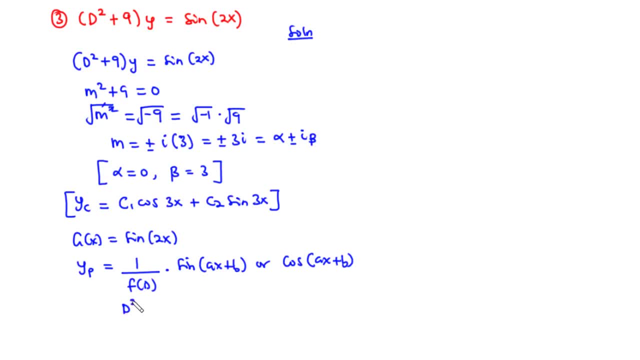 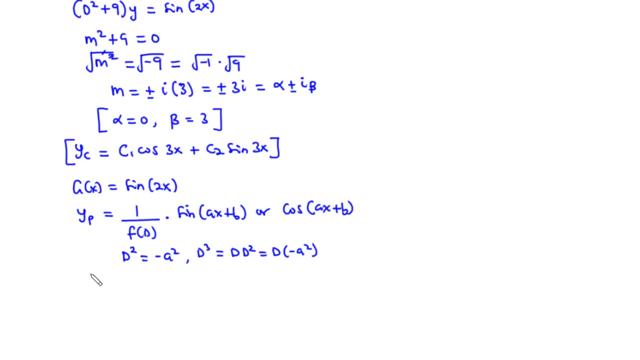 imply a sine of 2x, put, or we are going to put, such like: the square equals negative a square, the cube equals d, d square which is equal to d negative a square, and so on and so forth. now we have the coefficient of x here to be 2, therefore we have the value of a. 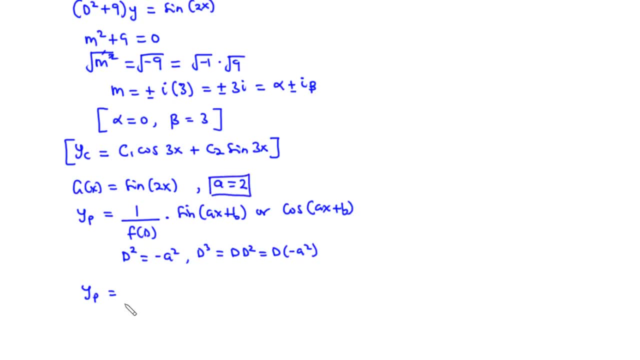 to be 2, so we are going to have y p equals 1 over now. we have f of d, f of d, here to be d square plus 9, so we have d square plus 9, and then times sine 2x, so this is equal to. we have 1 over now. d square is equal to. 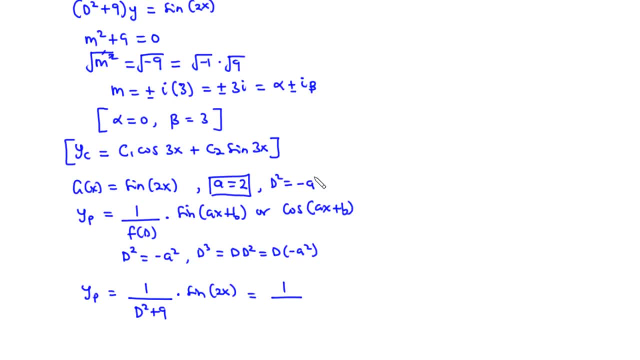 d square is equal to negative a square. now we have negative. sorry, we have a. we have a to be 2, so that is negative 2 square and that is equal to negative 4. we have a. we have d square to be negative 4, so we are going to have negative 4 plus 9 times sine 2x and that is equal to 1 over. 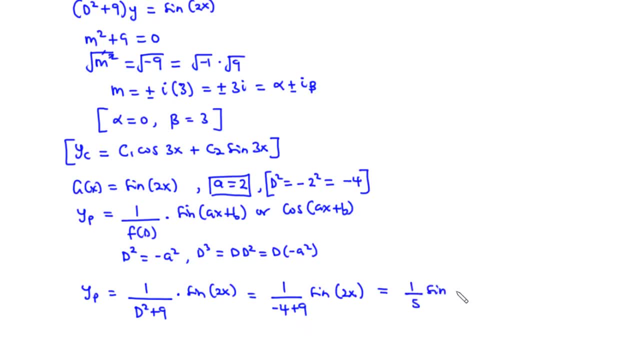 5 times sine 2x. so we have y p to be equal to 1 over 5 sine 2x. so that is the particular integral. therefore we have the general solution: y giving us c1 cos 3x plus c2 sine, 3x plus 1 over 5 sine. 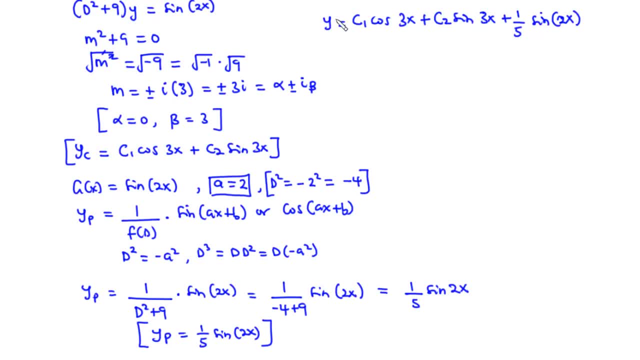 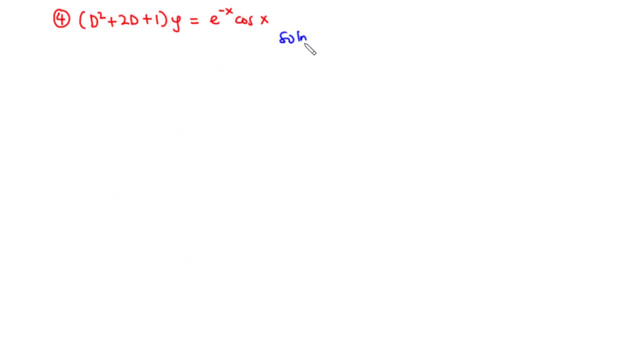 2x. so that is the particular integral. therefore we have c1 cos 3x plus c2 sine 3x plus 1 over 5 sine 2x. now to the last example. let's try to solve this differential equation as well. now to the last example. let's try to solve this differential equation as well. 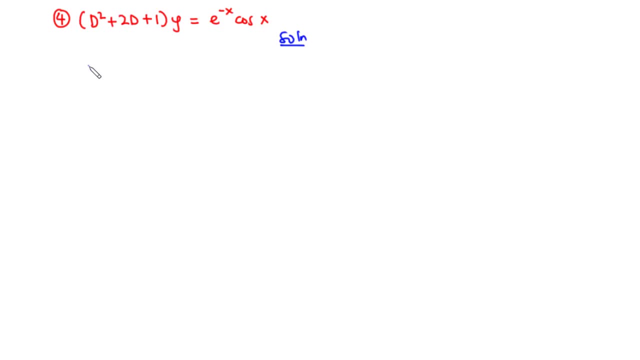 now to the last example. let's try to solve this differential equation as well. so, first of all, we, so, first of all, we so, first of all, we generate the auxiliary equation. that is, we have generate the auxiliary equation. that is, we have generate the auxiliary equation, that is, we have m square plus 2m. 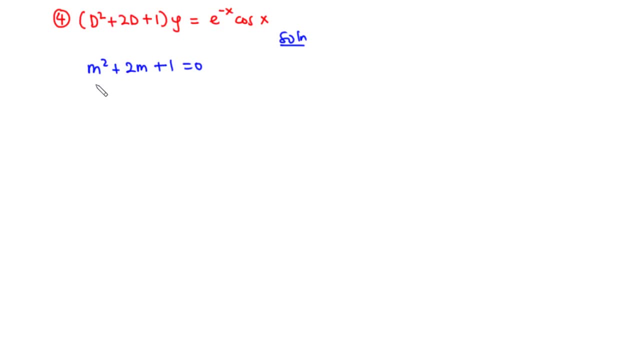 m square plus 2m. m square plus 2m plus 1 equals zero. now we have the plus 1 equals zero. now we have the plus 1 equals zero. now we have the coefficient of m squared to be one. coefficient of m squared to be one. 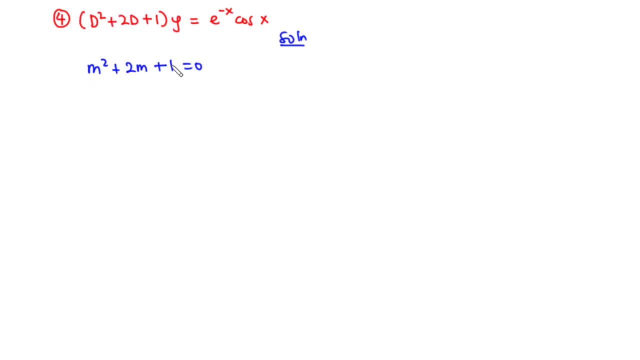 coefficient of m squared to be one. coefficient of constant term also to be coefficient of constant term also to be coefficient of constant term also to be one. so we want two values that when you one. so we want two values that when you one. so we want two values that when you multiply you have one when you add you. 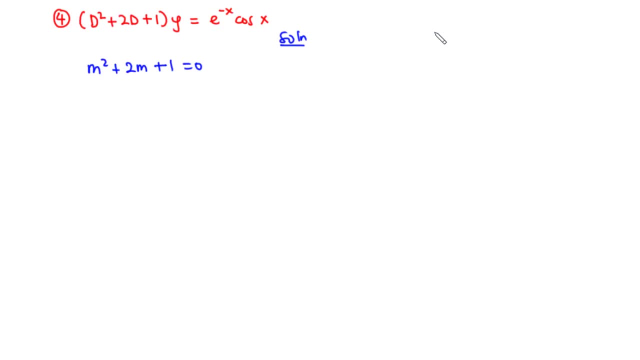 multiply, you have one. when you add, you multiply, you have one. when you add, you have two, that is one and then one. have two, that is one and then one. have two, that is one and then one. so this is going to be. so this is going to be. 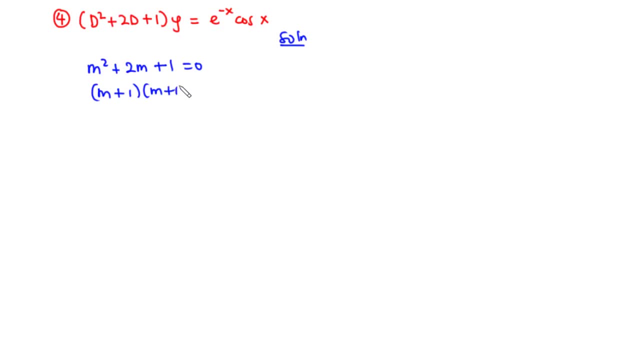 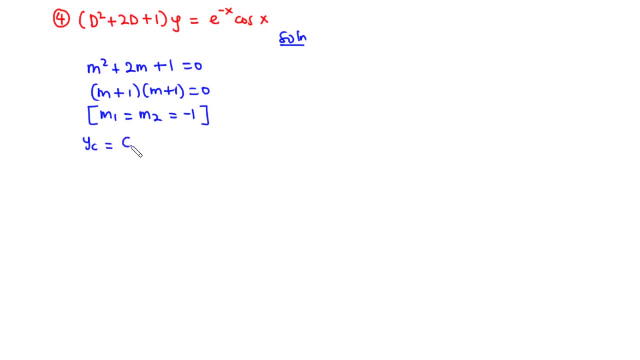 m2 and that is equal to negative one m2 and that is equal to negative one. therefore, we have yc, therefore we have yc. therefore, we have yc to be equal to c1 e to the power to be equal to c1 e to the power to be equal to c1 e to the power negative x plus. 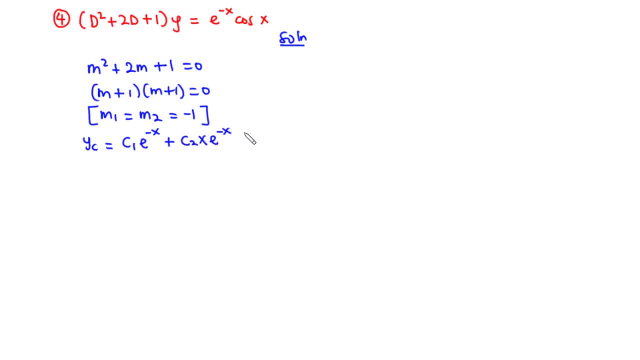 negative x plus negative x, plus c2, c2, c2, x e to the power negative x. this is the x? e to the power negative x. this is the x? e to the power negative x. this is the complementary, complementary, complementary function. now let's try to find the. 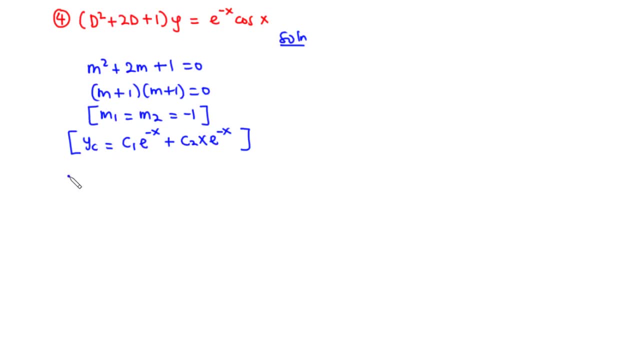 function now, let's try to find the function now. let's try to find the particular integral, particular integral, particular integral now with a particular integral, this time now with a particular integral, this time now with a particular integral. this time we have the product of two functions. we have the product of two functions. 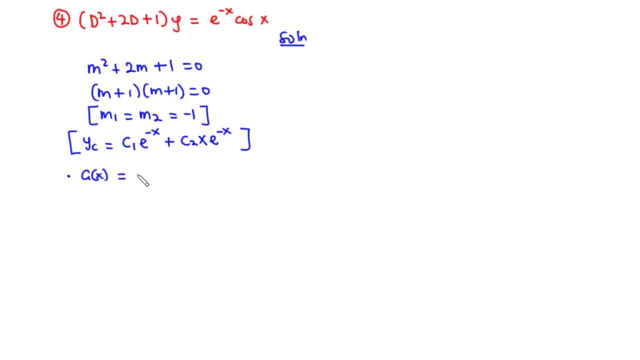 we have the product of two functions. we have g of x, we have g of x. we have g of x to be equal to, to be equal to, to be equal to x. so that is, you have e to the power, x. so that is, you have e to the power. 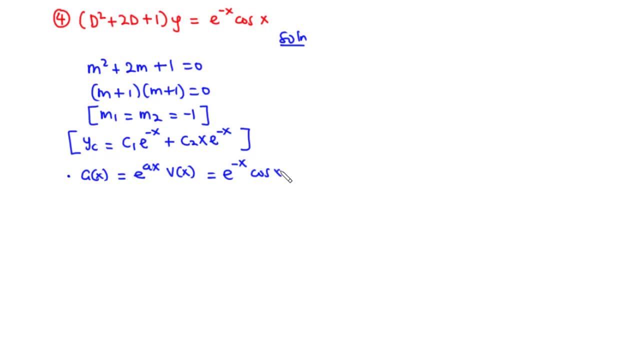 x. so that is, you have e to the power. negative x, negative x, negative x, times, times, times, cos x now. so long as you have the cos x now, so long as you have the cos x now, so long as you have the product of functions in this form, that 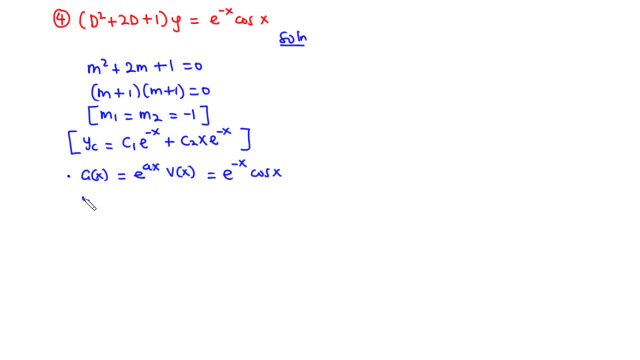 product of functions in this form. that product of functions in this form, that is e to the power a x times v of x is e to the power a x times v of x is e to the power a x times v of x. then we have the particular solution yp. 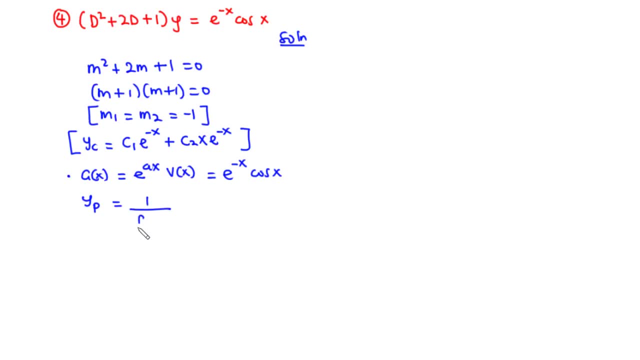 then we have the particular solution yp. then we have the particular solution yp equals equals, equals 1 over f of d, f of d, f of d, so f of d times, so f of d times, so f of d times e to the power a, x, v of x. so that will. 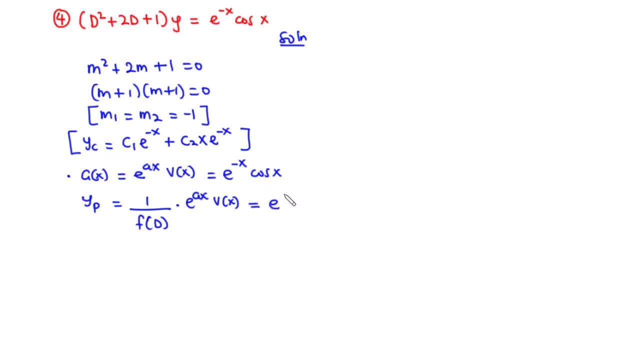 e to the power a x, v of x. so that will e to the power a x, v of x. so that will be equal to. you are going to shift, be equal to. you are going to shift, be equal to. you are going to shift. e to the power a- x on the left, and then 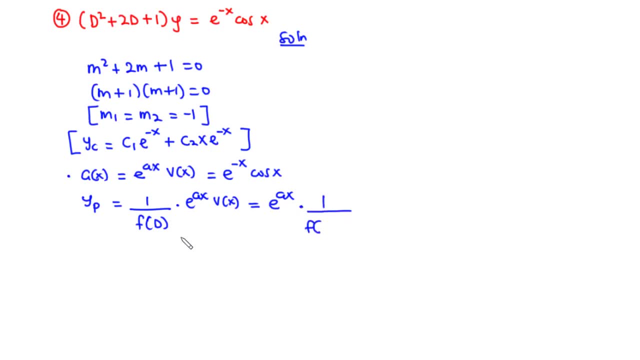 e to the power, a x on the left, and then e to the power, a x on the left, and then you have times one over. you have times one over. you have times one over. f of instead of f of d, you have f of d. f of instead of f of d, you have f of d. 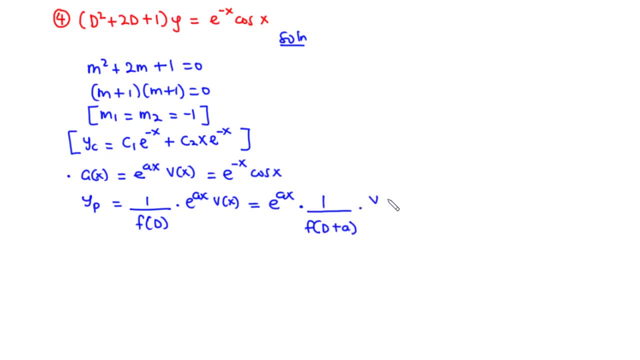 f of instead of f of d. you have f of d plus a plus a plus a, and then times, and then times and then times: v of v of v of of x, v of x, so of x, v of x, so of x, v of x. so here we have a comparing these two. 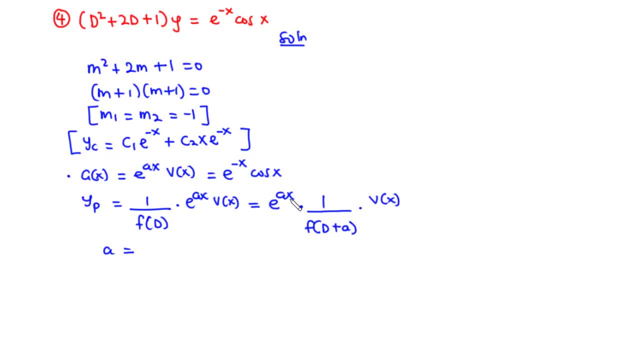 here we have a comparing these two. here we have a comparing these two functions, that is functions, that is, functions, that is, e to the power a x and then e to the e to the power a x and then e to the e to the power a x and then e to the power negative x. so e to the power a x. 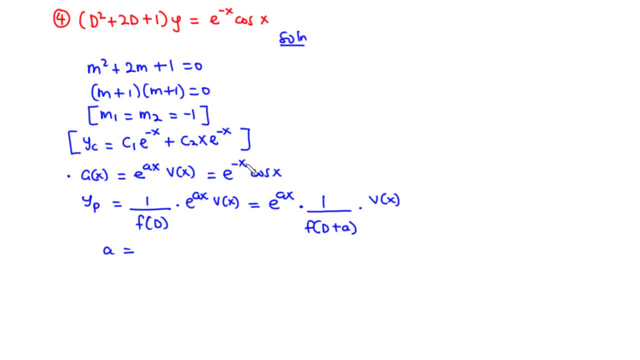 power negative x. so e to the power a x. power negative x. so e to the power a x and then e to the power negative x you and then e to the power negative x you and then e to the power negative x. you have the coefficient of x here to be. 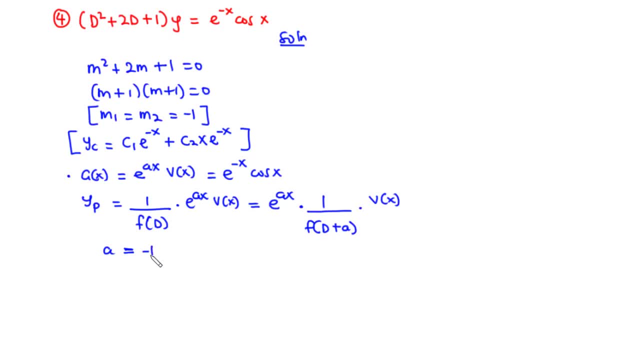 have the coefficient of x here to be. have the coefficient of x here to be negative one, so a is equal to negative one. so a is equal to negative one. so a is equal to negative one. negative one, negative one. and then, and then, and then, you have d plus a to be. 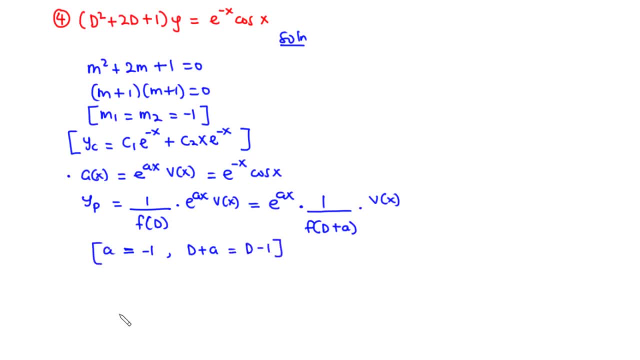 you have d plus a to be. you have d plus a to be: d minus one, d minus one, d minus one. therefore, we are going to have y p. therefore we are going to have y p. therefore we are going to have y p equals, equals, equals. we have e to the power, a x, so e to the 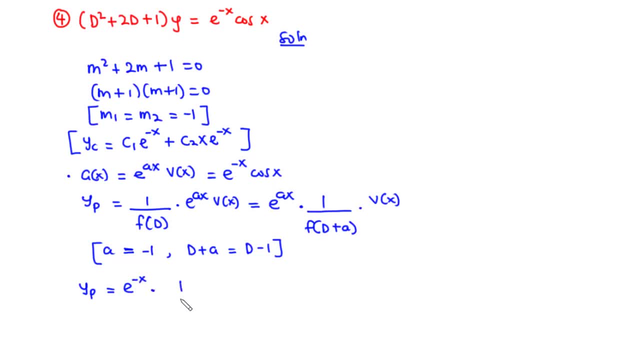 we have e to the power, a x, so e to the. we have e to the power, a x, so e to the power. negative x, power, negative x, power, negative x times. we have one over times. we have one over times. we have one over f of d. 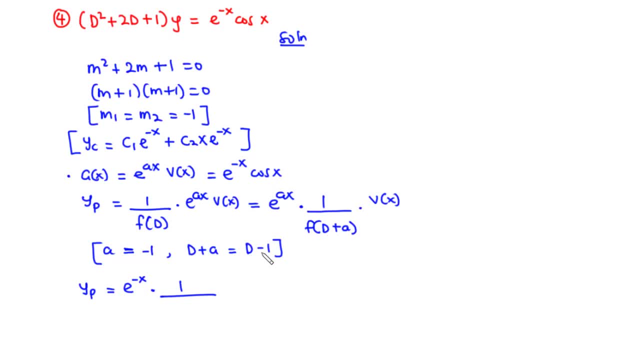 f of d, f of d plus a. so we are going to substitute plus a. so we are going to substitute plus a. so we are going to substitute d minus one, d minus one, d minus one in place of d, in place of d in place of d in here. so we are going to have d. 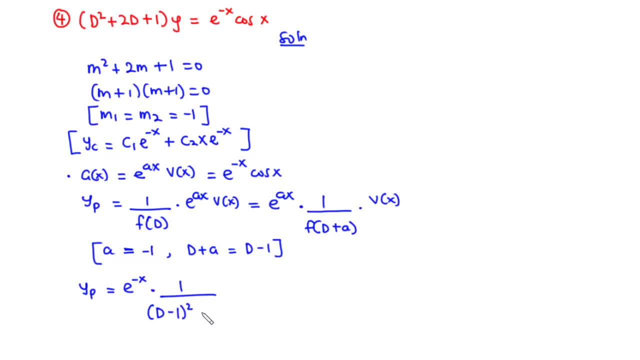 in here. so we are going to have d in here. so we are going to have d minus one minus one minus one all square plus two into bracket d minus all square plus two into bracket d minus all square plus two into bracket d minus one, one one plus one. 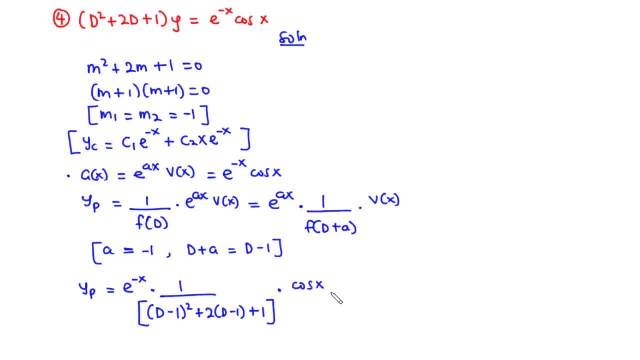 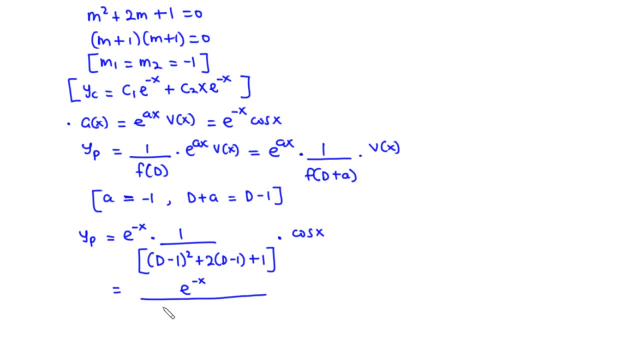 times v of x, which is times v of x, which is times v of x, which is cos x, so cos x, so cos x. so this becomes, this, becomes, this, becomes e to the power negative x, e to the power negative x, e to the power negative x. over here we have. 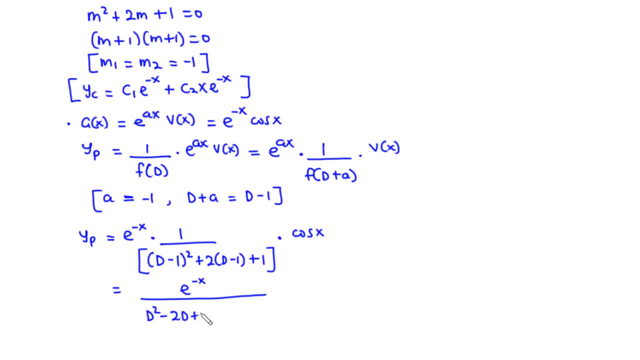 over here. we have over here, we have d square, d square, d square. minus, minus, minus, minus, minus 2d plus 1, and then plus 2d plus 1, and then plus 2d plus 1, and then plus 2d minus 2. 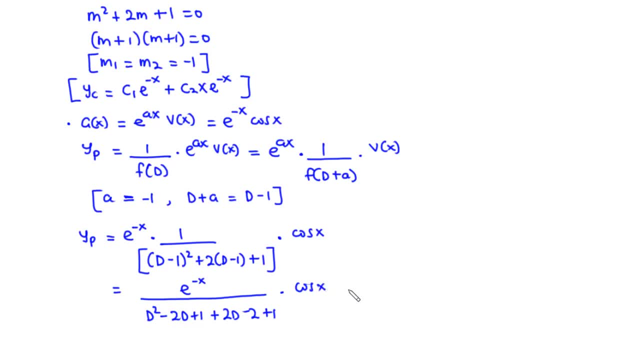 2d minus 2. 2d minus 2 plus 1 times plus 1 times plus 1 times cos x. now we have this equals cos x. now we have this equals cos x. now we have this equals. here we have. here we have. 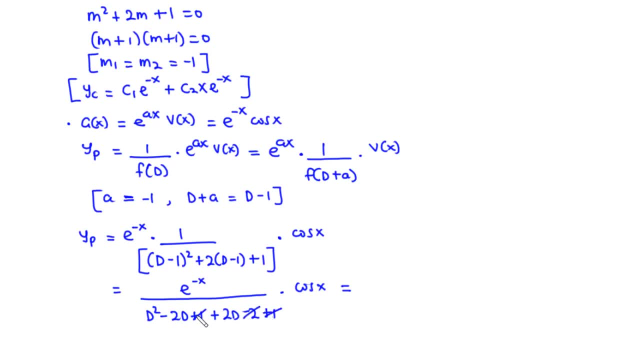 here we have plus one plus one, which is two, and then plus one plus one, which is two, and then plus one plus one, which is two, and then minus two. so they cancel out minus two, so they cancel out, minus two, so they cancel out. we have negative 2d, and then 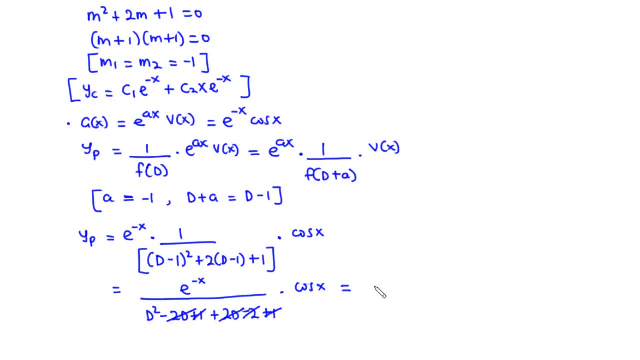 we have negative 2d and then we have negative 2d and then plus 2d- they also cancel out. so we plus 2d, they also cancel out. so we plus 2d, they also cancel out. so we have e to the power, negative x. 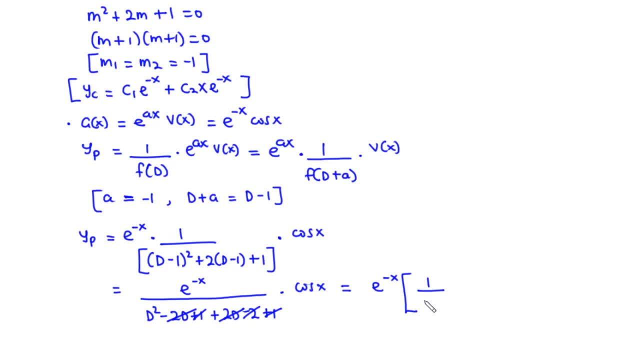 have e to the power negative x, have e to the power negative x times one over times one over times one over d square of cos x, of cos x, of cos x. so how do we simplify this? so how do we simplify this? so how do we simplify this? now, this is equal to e to the power. 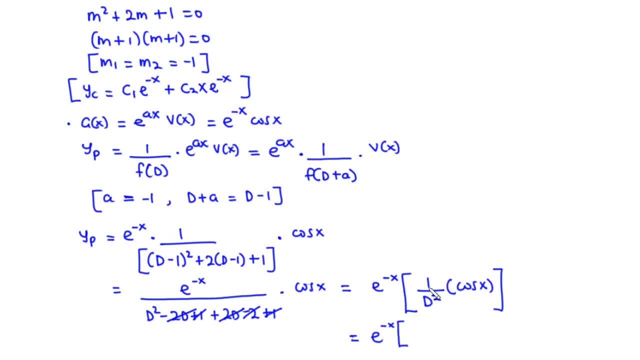 now this is equal to e to the power. now this is equal to e to the power. negative x, negative x, negative x, and then we have this is, and then we have this is, and then we have this is 1 over d square. so you can express this: 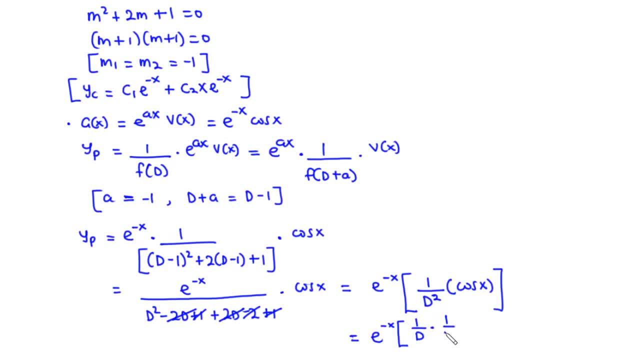 1 over d square. so you can express this: 1 over d square. so you can express this as: 1 over d, as 1 over d, as 1 over d times times times: 1 over d, 1 over d, 1 over d of cos x. 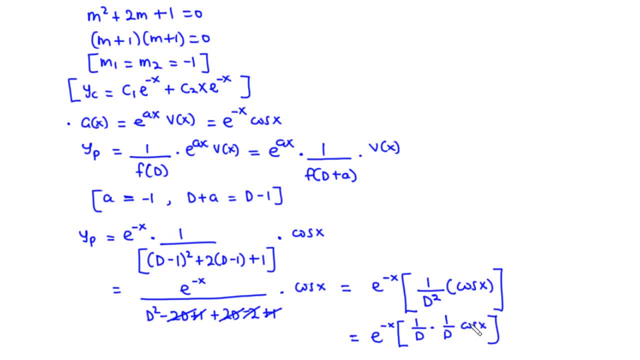 of cos x, of cos x. so this means that you are going to. so this means that you are going to. so this means that you are going to integrate, integrate, integrate the function cos x. you are going to the function cos x. you are going to the function cos x. you are going to integrate the function cos x. 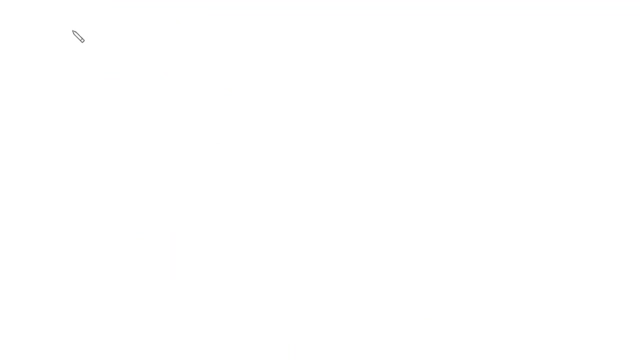 integrate the function cos x. integrate the function cos x. so we are going to have, so we are going to have. so we are going to have yp, yp, yp. we are going to have yp. we are going to have yp. we are going to have yp. equals, equals e to the power negative x. 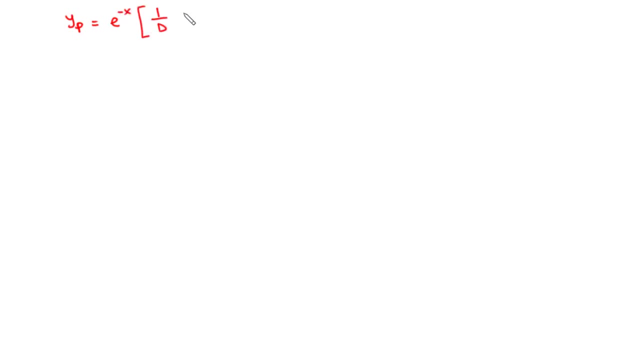 equals e to the power negative x, equals e to the power negative x. then into brackets. we have 1 over d. then into brackets we have 1 over d, then into brackets we have 1 over d. and then times the integral of and then times the integral of. 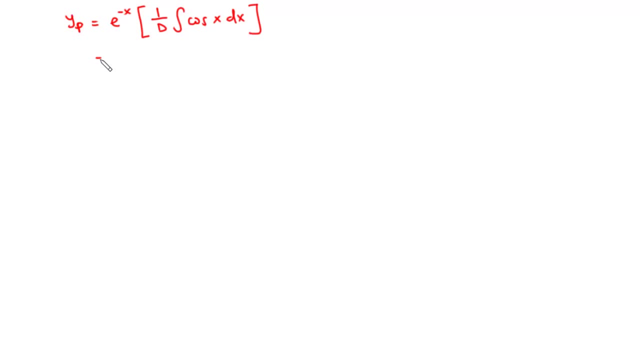 and then times the integral of cos x, cos x, cos x, dx, so that becomes e to the power negative x, so that becomes e to the power negative x, so that becomes e to the power negative x, and then you have 1 over d, and then you have 1 over d. 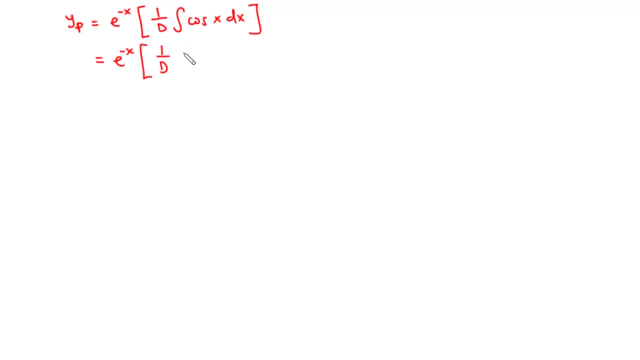 and then you have 1 over d off now when you integrate cos x, you have off. now, when you integrate cos x, you have off. now, when you integrate cos x, you have sine x, sine x, sine x, so sine x, so sine x, so sine x, and then it means that you are going to 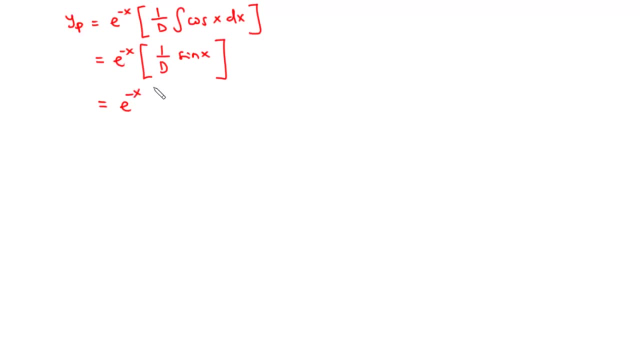 and then it means that you are going to, and then it means that you are going to also integrate sine x. so you have e to also integrate sine x. so you have e to also integrate sine x. so you have e to the power negative x, the power negative x. 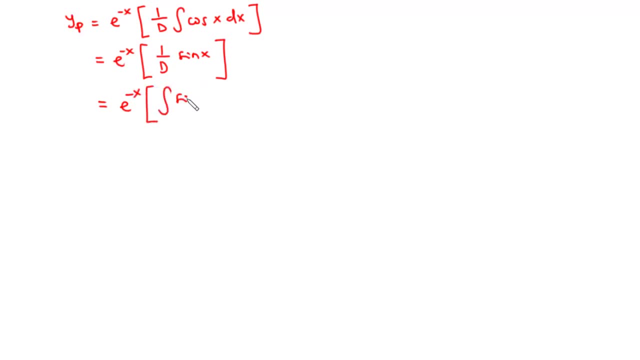 the power negative x times the integral of sine x, sine x, sine x, dx, dx, dx. now, if you integrate, now if you integrate sine x, then you have negative sine x, then you have negative sine x, then you have negative cos x, cos x, cos x, so this becomes negative. 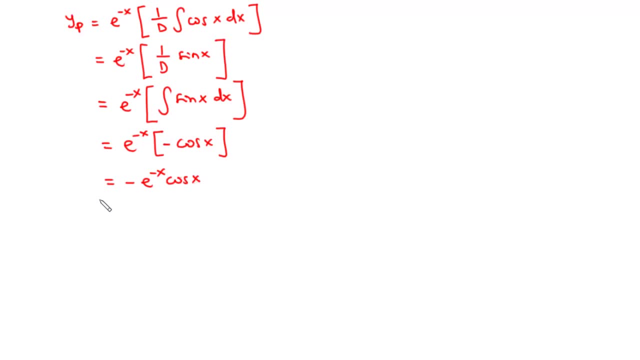 so this becomes negative. so this becomes negative. e to the power negative, x. e to the power negative, x. e to the power negative. x cos x, so that is yp, cos x, so that is yp, cos x, so that is yp. therefore, we have the general solution y. 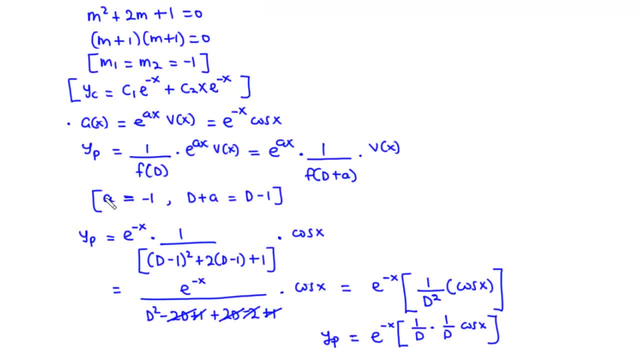 therefore, we have the general solution y. therefore, we have the general solution y to be equal to. we have yc to be c1 e to the power. we have yc to be c1 e to the power. we have yc to be c1 e to the power, negative x plus c2 times x. 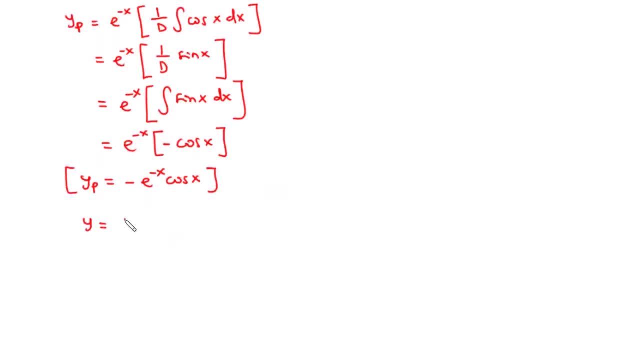 negative x plus c2 times x. negative x plus c2 times x times e to the power negative x times e to the power negative x times e to the power negative x, so c1 e to the power negative x, so c1 e to the power negative x. 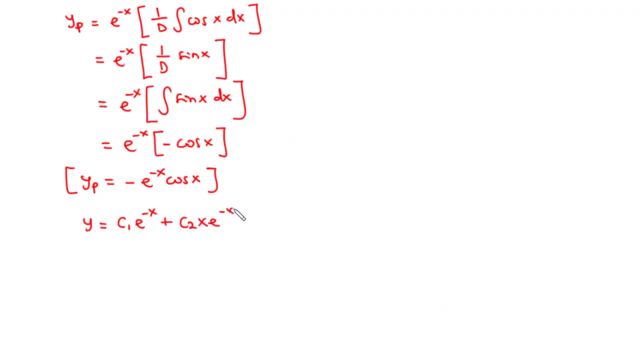 so c1 e to the power negative x plus c2 x e to the power negative x plus c2 x. e to the power negative x plus c2 x. e to the power negative x minus minus minus e to the power negative x e to the power negative x. 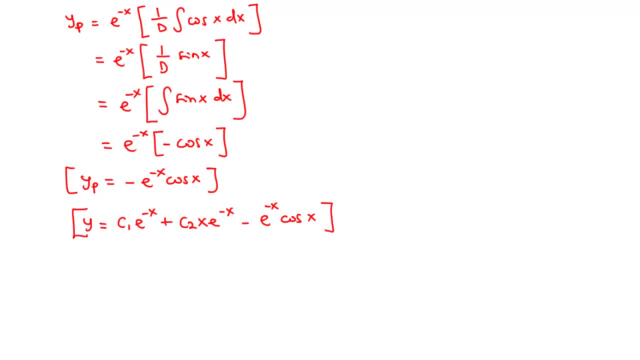 e to the power negative x cos x. 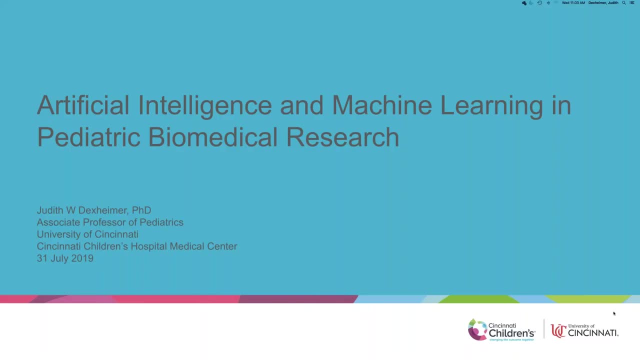 Good morning and welcome to the AWS Education Research Seminar Series. This morning we're going to be discussing artificial intelligence and machine learning in pediatric biomedical research with Professor Judith Dexheimer. Dr Dexheimer is an associate professor of pediatrics at Cincinnati Children's Hospital Medical Center and the University of Cincinnati.